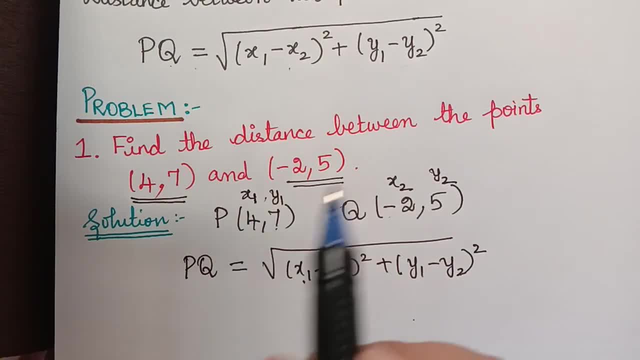 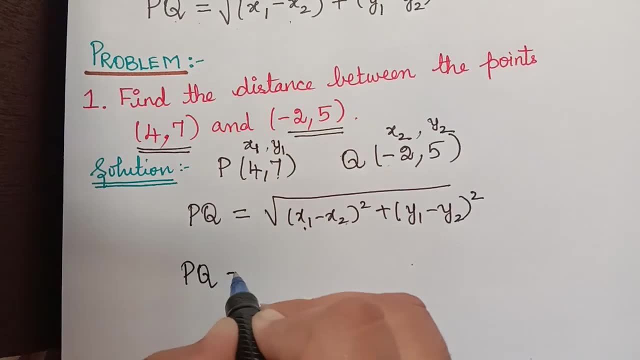 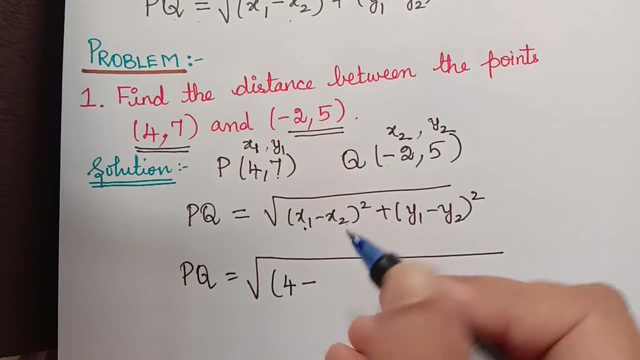 2, so this coordinate is x 1 comma y 1. this is x 2 comma y 2, so let us substitute that now here. so therefore p q will be equal to 0.2 root of now. what is x1, 4, so 4 minus. what is x2 minus 2, so 4 minus of minus 2, the whole square. 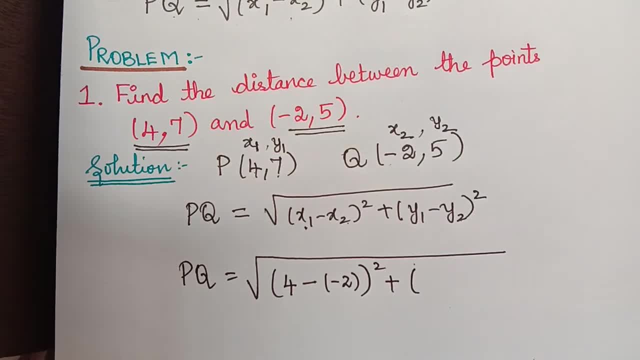 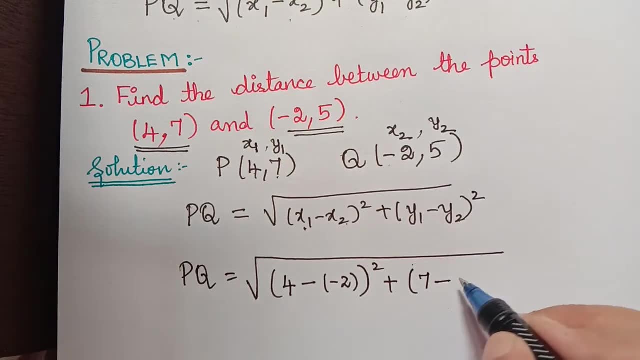 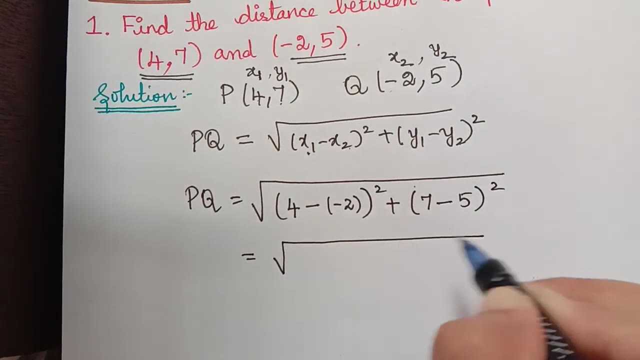 plus what is y1. y1 is 7, so 7 minus what is y2, it is 5, so 7 minus 5, the whole square. so let us simplify this so that is equal to square root of now. this will be 4 minus of minus 2, so 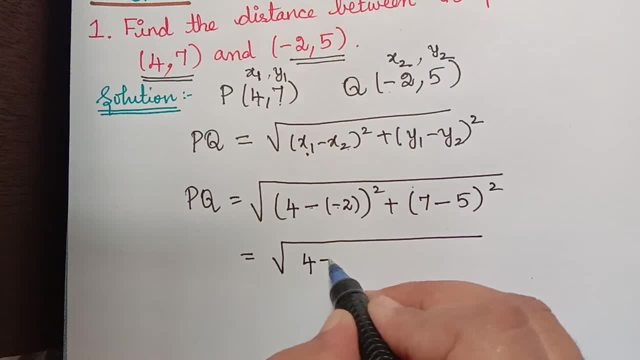 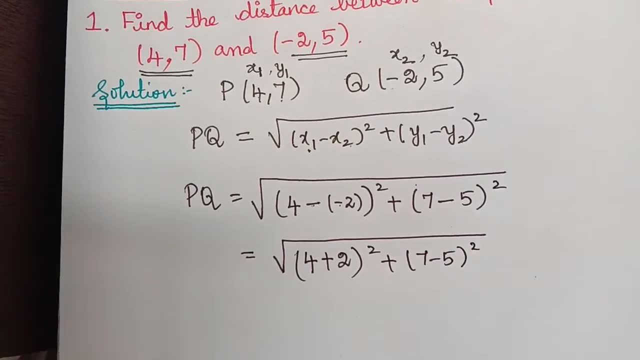 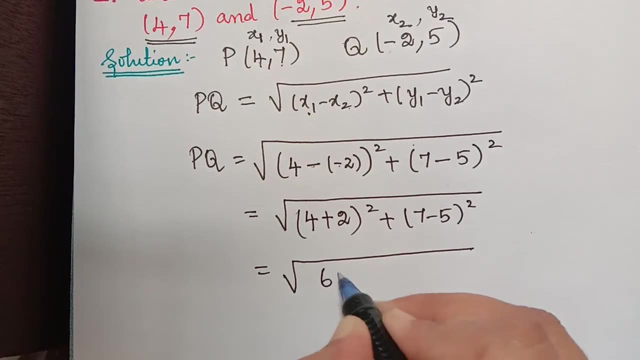 minus, multiplied with minus will become positive, so plus. so 4 plus 2, the whole square, plus 7 minus 5, the whole square. further simplifying this, we get so this is to be equal to square root of 4 plus 2, that is, 6 square plus 7 minus. 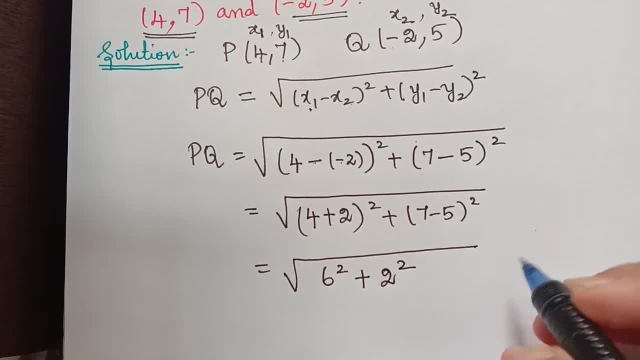 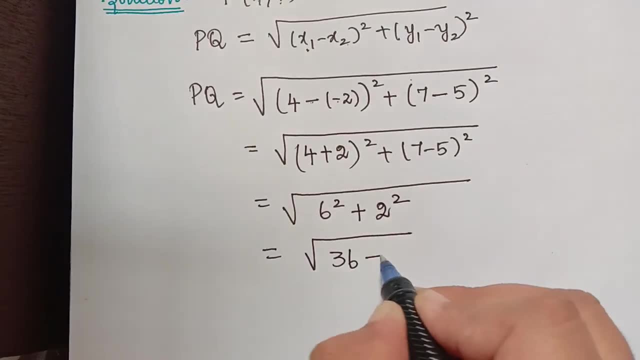 bar. So this will be equal to 6 square plus 7 minus 5, the whole square. so that is easier to missing 5: 2 square and so that will be equal to square root of now. what is 6 square? it is 36 plus 2. 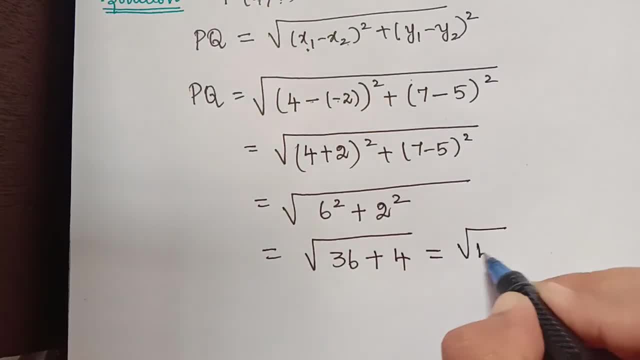 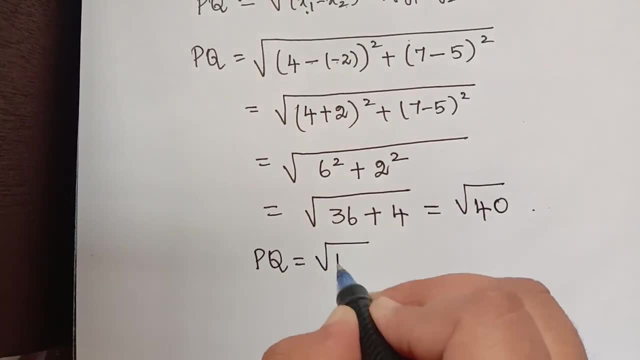 squared is 4, so that is equal to square root of 40. so therefore the distance between the point p and q is equal to square root of 40. now, because units are not given in the question, we can generally write it as square root of 40 units. so this is the answer. we can further simplify. 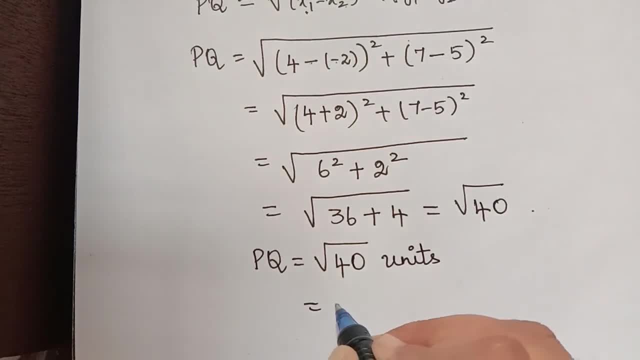 this because square root of 40 can be actually written as square root of 4 multiplied with 10. now what is the square root of 4? it is 2, so that is equal to 2 square root of what is left out, because we have taken this 4 out of the square root and it has become 2 square root of 10 will. 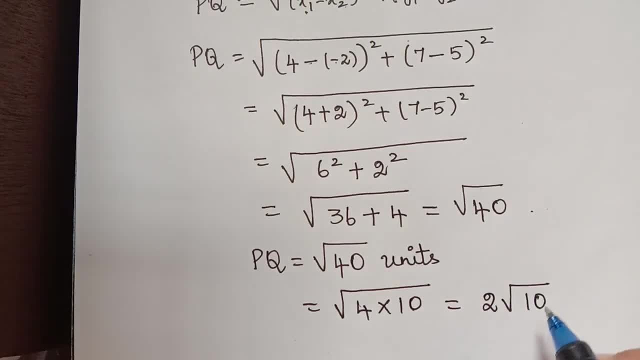 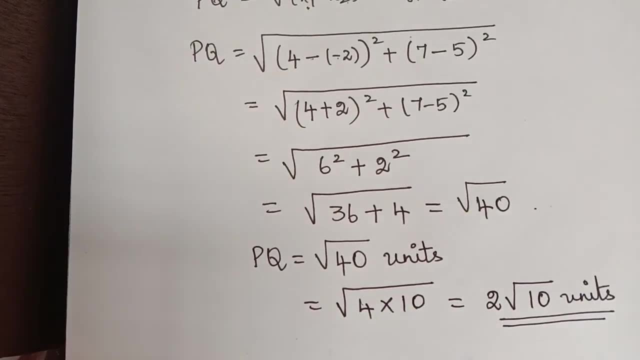 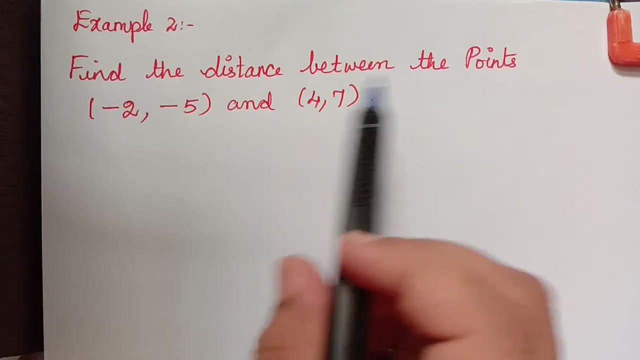 be remaining. So we have 2 square root of 10 units. so this is the distance between the point p and q. hope you have understood this. let me explain this with the help of another one more example. now here we have another one example. so now here we have two points and we have to find the distance between these. 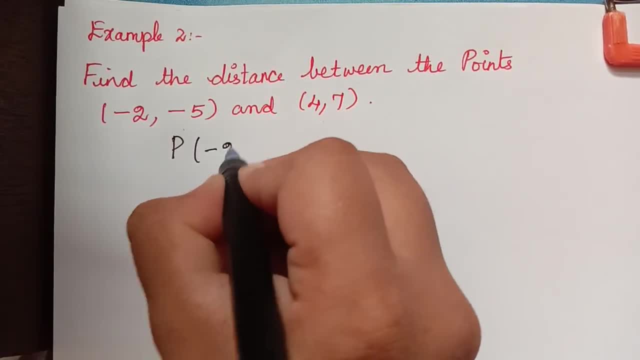 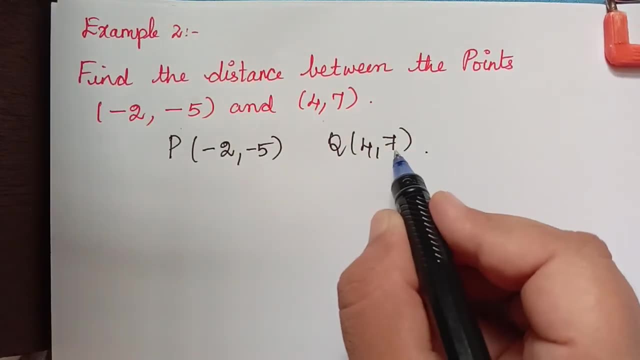 two points. so let us take the point p as minus 2 comma minus 5, and the point q as 4 comma 16, and we have to find the distance between these two points. so let us take the point p as minus 2, 7. now we have to find the distance between these two points, which is given by the formula pq is: 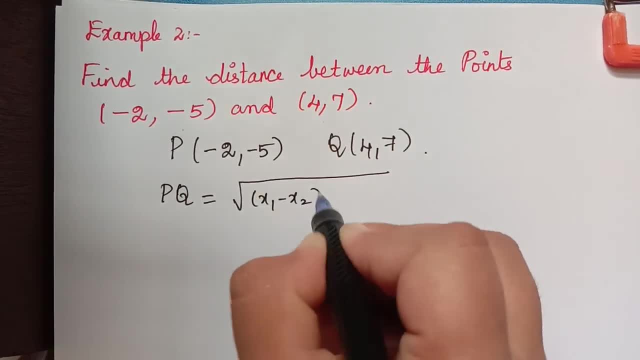 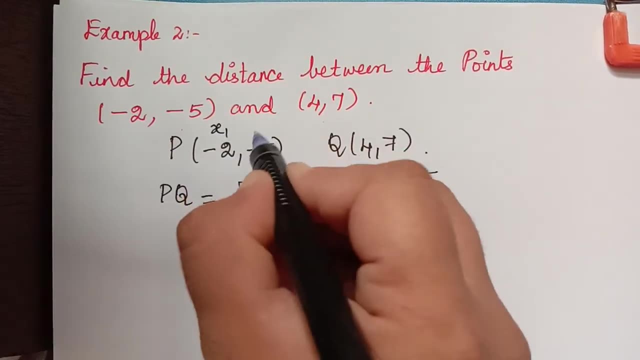 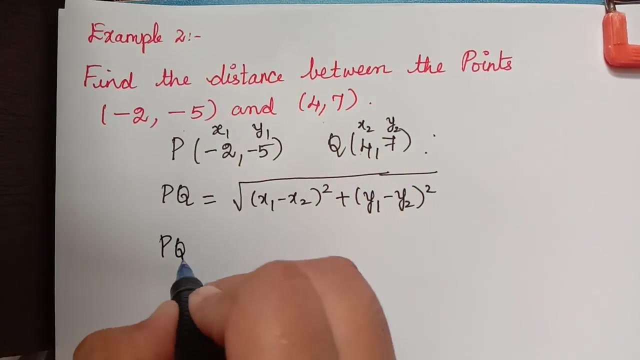 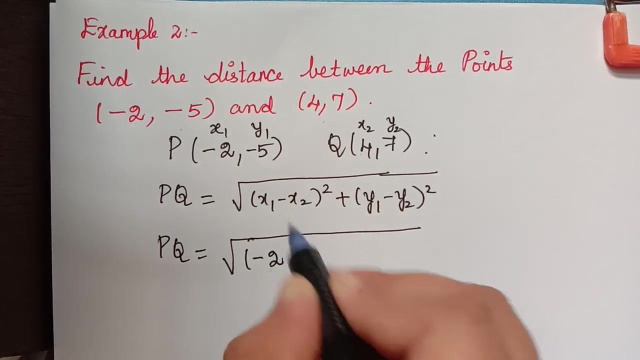 equal to square root of x1 minus x2, the whole square. plus y1 minus y2, the whole square with this is x1, y1 and this coordinate is x2 and this is y2. so now we shall substitute here, so pq will be equal to square root of now. what is x1? it is negative 2. so minus 2 minus x2 is 4 the whole. 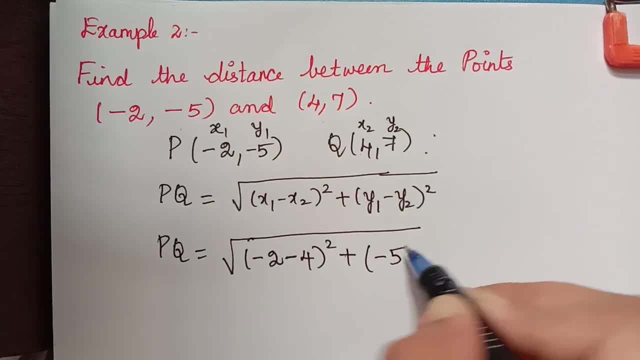 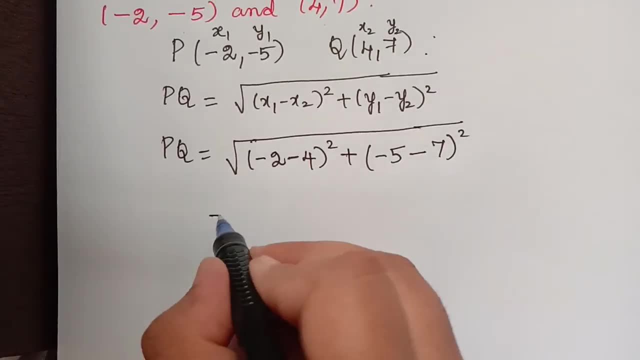 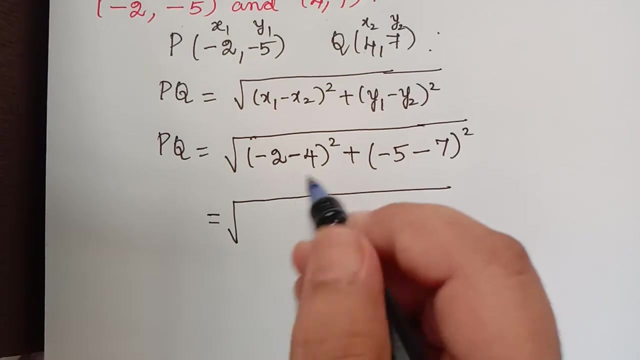 square: plus y1 is minus 5, minus y2 is 7, so 7 the whole square. so this will be equal to square root of what is minus 2 minus 4, so negative 2. negative 4 is negative 6, so negative 6 the whole square. 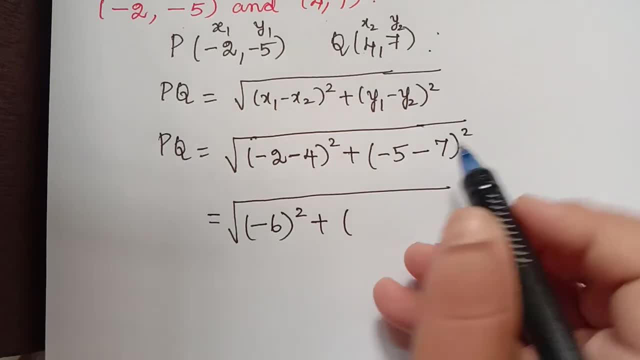 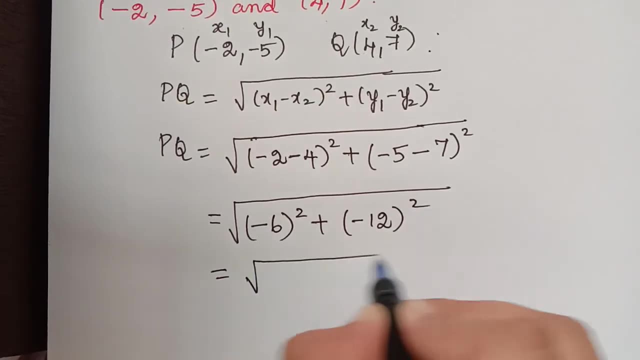 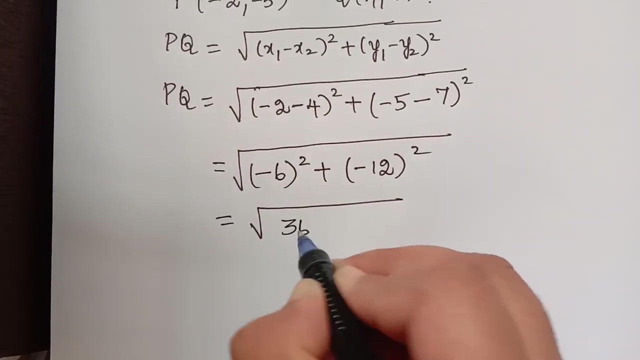 plus negative 5. negative 7 is negative 12. so minus 12 the whole square. so now this can be simplified further. so that is equal to square root of what is minus 6. the whole squared it is 36. anyway, minus into minus will become plus, so it becomes positive. 6, 6 times is 36 plus. 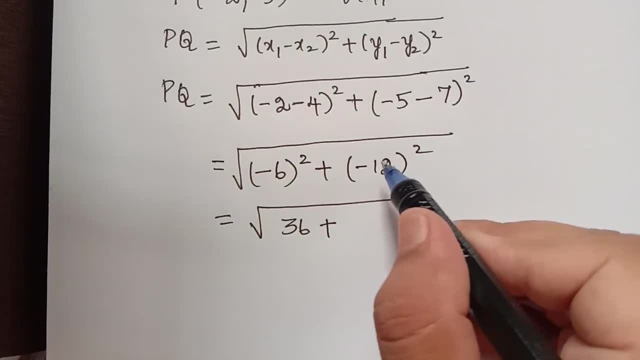 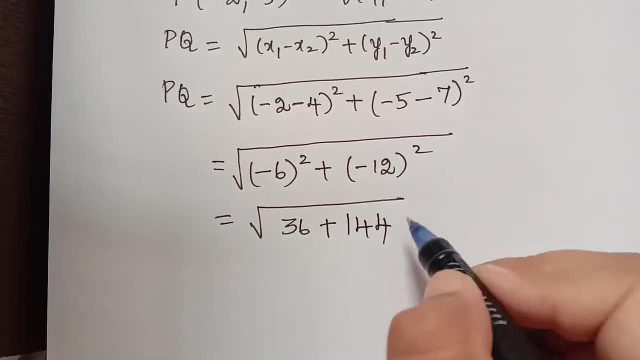 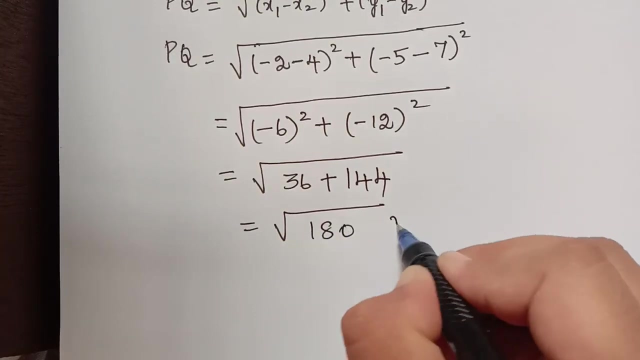 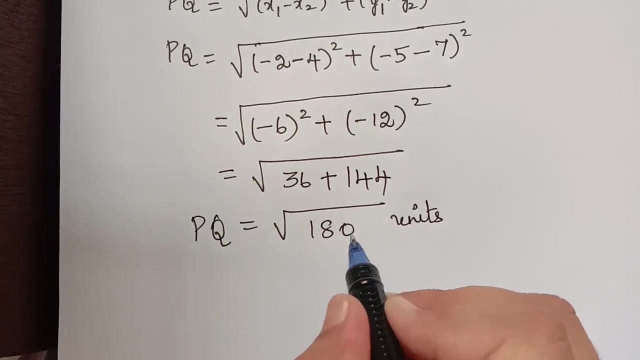 now here we have minus 12. the whole squared, so it is minus into minus, will become positive, and 12 12 times is 144. so we get this. so that is equal to square root of what is 36 plus 144. it is 180 units. so therefore the distance between the points p and q is square root of 180 units. you. 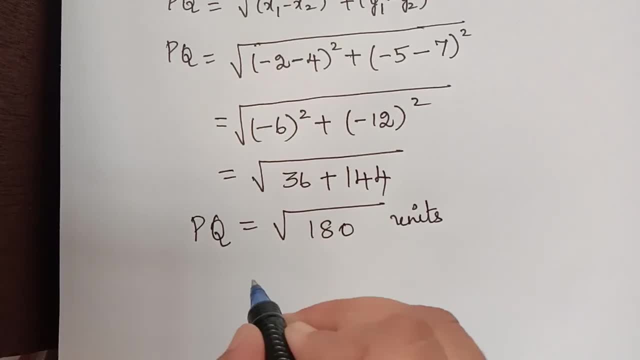 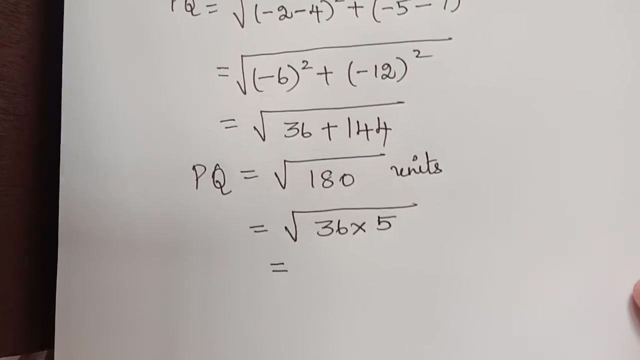 can leave it as such, or you can simplify this even more. so how can we simplify this? this 180 can be written as 36 multiplied with 5, because 36 multiplied with 5 gives us 180, and so this 36 can be written as i mean, because it is. 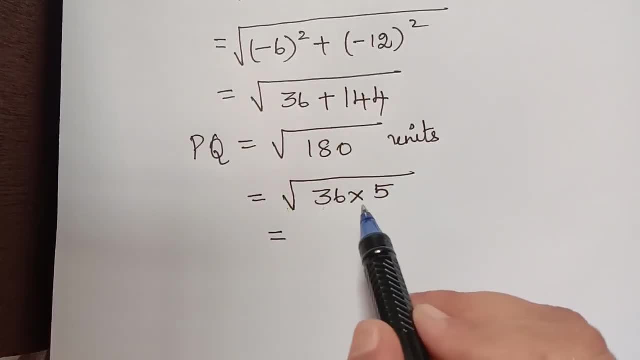 inside the square root. this is square root of 36 multiplied with 5. so when we take out 36 out of the square root, it becomes 6, because we know that 6- 6 are 36 and so square root of 36 can be written.